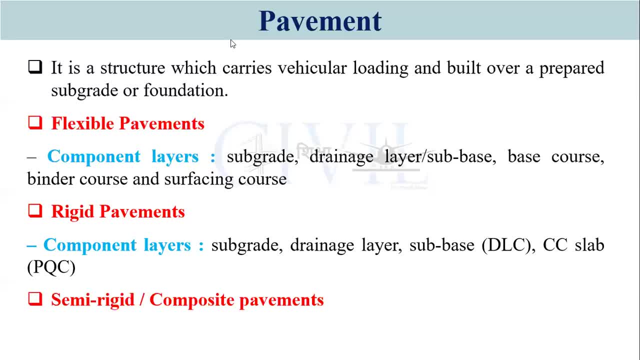 we do have the combination of rigid pavement and flexible pavement, which is called as the semi-rigid or composite pavement. So in general, the pavement is a structure which is designed to carry the vehicular load and also it is constructed over a prepared subgrade or foundation and it is the structure 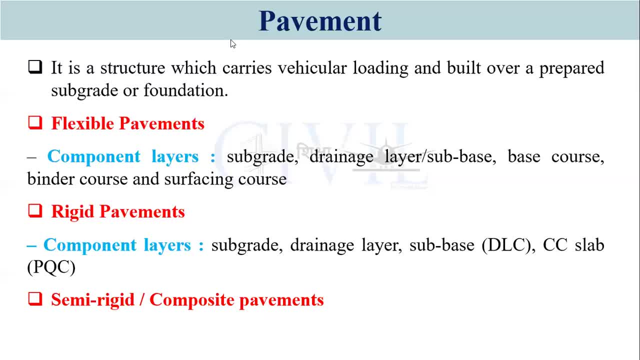 which has many layers or multiple layers. So that is why we also call pavement as a multilayer structure. and this multilayer structure means nothing but the structure which is constructed using these different types of layers. Here I have mentioned total 5 layers. so this is: 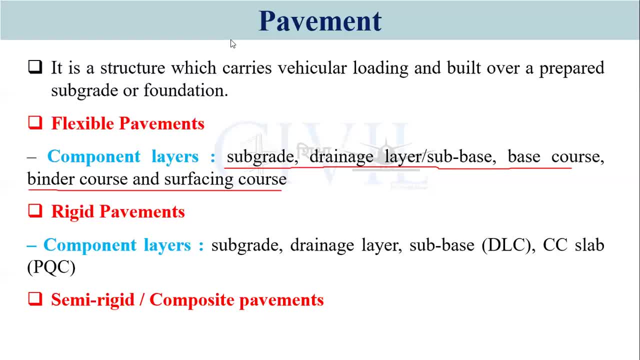 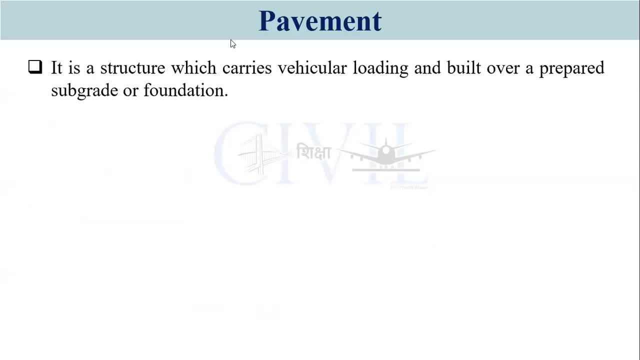 nothing but a 5 layer structure. so this is nothing but a multilayer structure. In the next slide we are going to discuss about the structure. We are going to discuss about the different component of a flexible pavement. so again, you can read the same definition over here: 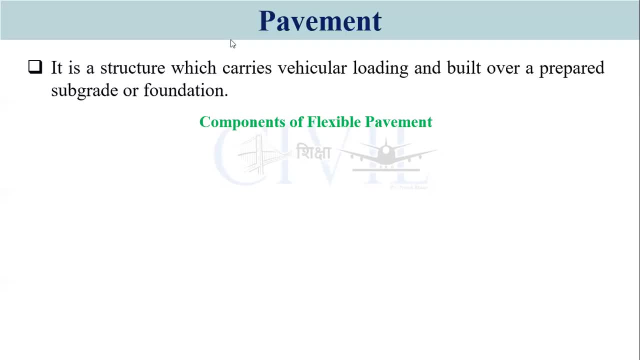 but here we are going to discuss the components of a flexible pavement. so when you talk about a flexible pavement, what do we have? so, number one, the foundation or natural subgrade. so the natural subgrade is nothing, but it is a layer of the material which is present in the on the you. 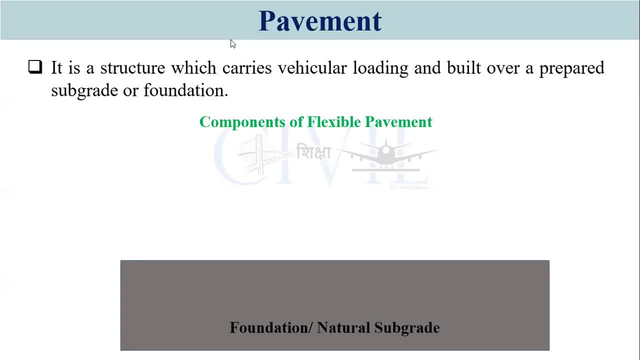 can say it is a layer of parent material. so suppose if i am going to construct a road in mumbai, then i will get a red color soil, or say the red soil, where at the same time, if i will go to another region of malaysia i might get the black cotton soil. so in simple words, if i am 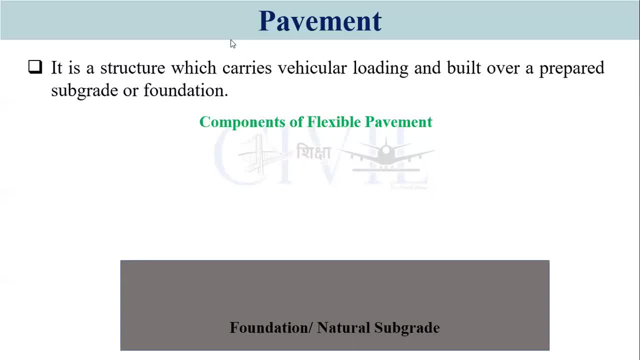 going to construct one layer of the parent material. that layer is going to simply called as the foundation or natural subgrade. but what happens? generally, the strength of that parent layer, or, sorry, strength of the parent material, is not that much good. so for that, what we have to do, we have to compact our subgrade or we have to increase the strength of our subgrade. 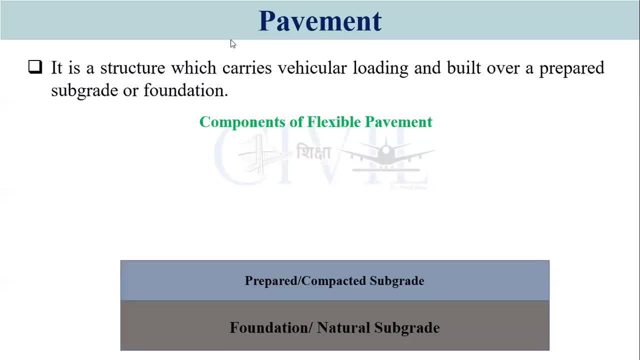 and to increase the strength of our subgrade. what we do, we prepare or we compact the subgrade. so by doing this, what we are doing, whatever is the strength of this parent material, what we are going to do, we are going to increase the strength. how we are going to strength increase, how we are. 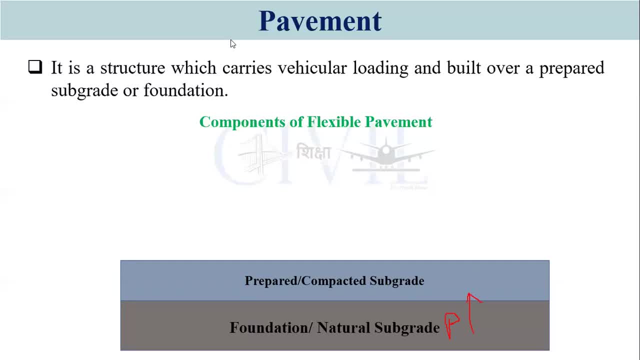 going to increase the strength by compacting this subgrade, or which is also called as the prepared subgrade, and in general, the thickness of this layer is 500 millimeter as per irc 37, but the thickness of this layer is infinite. the bottom most layer, the thickness of 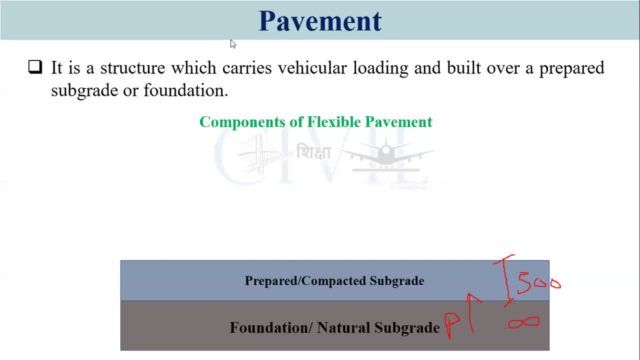 this layer is infinite, this thing you have to keep in mind. the thickness of compacted subgrade is always 500 millimeter, whereas the thickness of natural subgrade is infinite. then, after that, we are having another layer, which is called as the sub base or generally granular sub base. so this 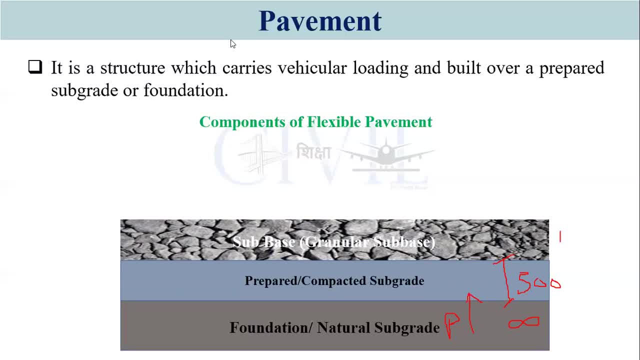 is the third layer from the bottom which is generally provided for drainage purpose in any pavement, whether it is rigid pavement or flexible pavement. so this is the third layer from the bottom, and this third layer is for drainage purposes in any pavement or for designated pavement. so for 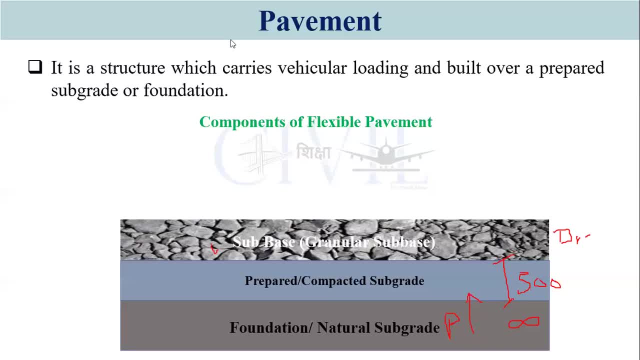 drainage purpose. we do provide this layer. you can see all the granular materials are present, to say, all the aggregates are present over here. that's why this layer is simply called as the granular sub base. after this we are going to have another layer which is called as the base course and is 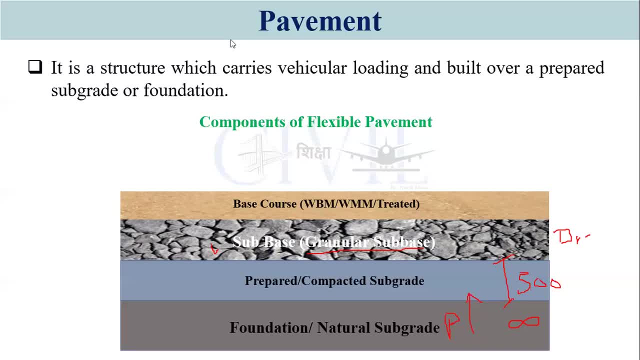 there. this base course can be a wbm or a treated base course. so wbm means water bount. i introduce are against the water-, далее brat material which is treated with cement, lime or fly ash and after that we are going to. 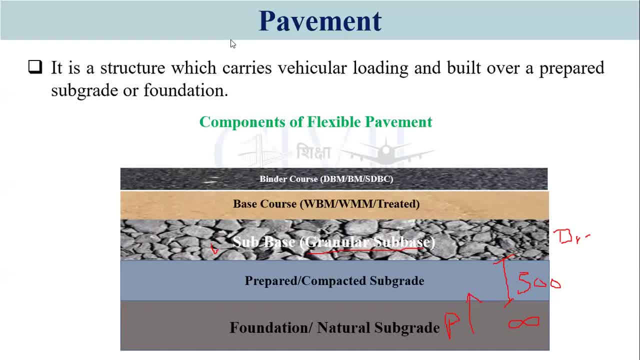 have one more layer, which is called as the binder core. So here what you have to understand: that these layers are also called as the granular layer or unbounded layer. Why? Because we are not going to use any binding material in this layer. 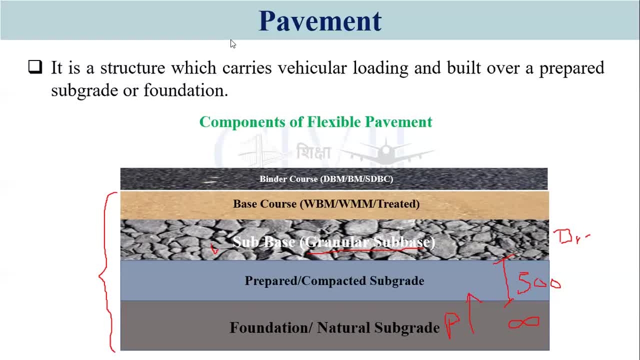 These are the same layer which are prepared using normal earthen material. But when we prepare the same layer by using any binder material or say any bituminous material, then that layer is going to call as the bituminous layer. So that I am going to explain in the next figure. 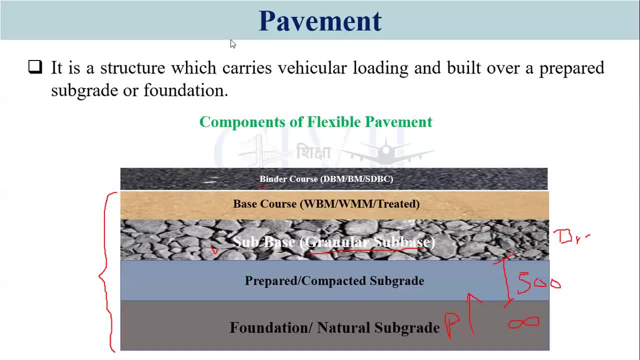 So here, after the base course, we are going to provide another course which is called as the binder course, and the binder course may be DVM, which is dense bituminous macadam, BM, which is, which means bituminous macadam, or SDBC, which means semi dense bituminous. 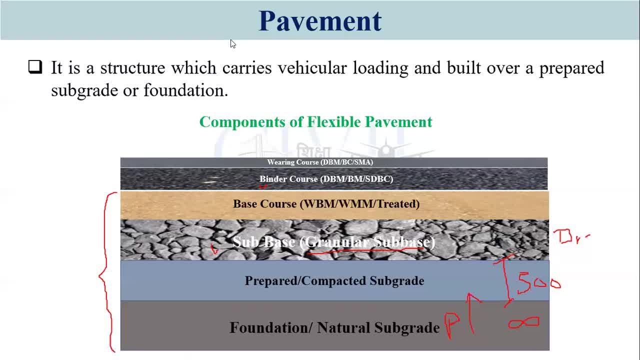 concrete. And in the last, In the, on the bottom, On the top, we are going to have the veering course, or say the surface course, which can be DVM, which is, I have already told you, dense, bituminous. macadam or BC means bituminous. 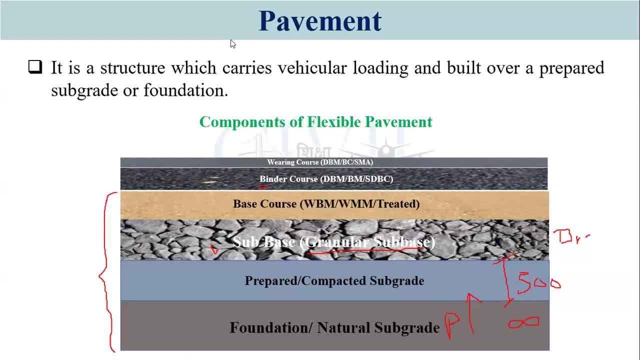 concrete, or SMA means stone mastic asphalt. So these are the different layer which we do generally construct- sorry, which we generally provide in a flexible pavement. These layers are called as the granular layer, whereas these top two layers are called as the bituminous layer. 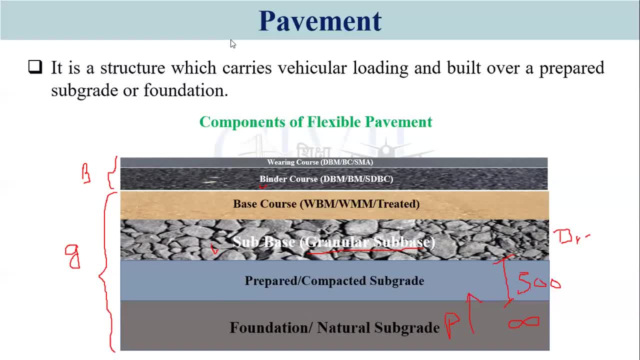 So this is the difference that you have to understand. This is the first set of layer, Which are the bituminous layer, and this is the second set of layer, which are your granular layer. Now, other thing that you would understand over here, that whenever we construct any flexible 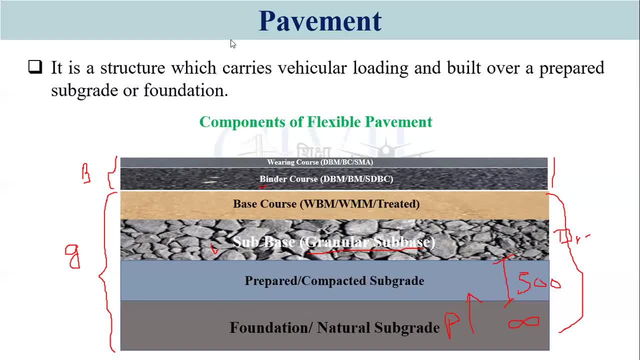 pavement in between a veering course and a base course, we generally provide a binder course. So this is a binder course which is provided between a bituminous layer and a non bituminous layer At the same time. what we do, we provide a thin coat of bitumen also, this thin coat of bitumen. 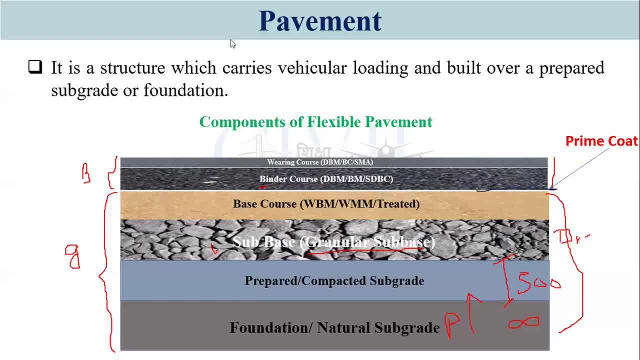 is provided in between a granular material Right. So this is a bituminous layer and a bituminous layer. So whenever you are going to lay a bituminous layer over a granular layer, what you will do? you will apply a thin coat, or say thin spray of bitumen, so that the binding will be proper. 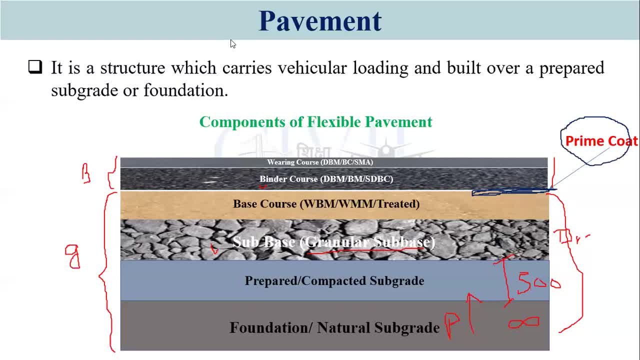 and that coat is simply called as the prime coat. At the same time, when you're going to lay a bituminous layer or another bituminous layer that you can see over here, this is a bituminous layer, Right, And we are going to provide another bituminous layer over here. 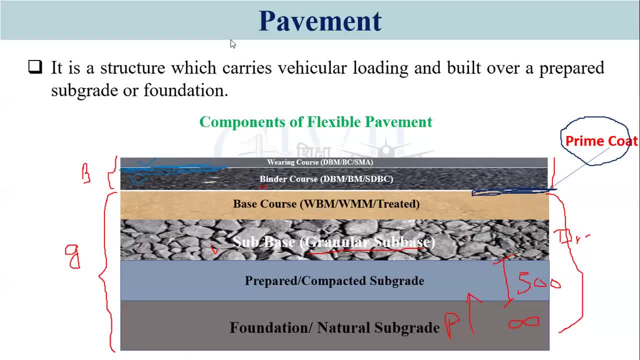 So in between. So we are going to provide one thin coat of bitumen over here, and that thin coat of bitumen is simply called as the take coat. So there are different components that you can simply see over here, which are nothing but your, first of all, your natural subgrade or foundation. then you are going to provide 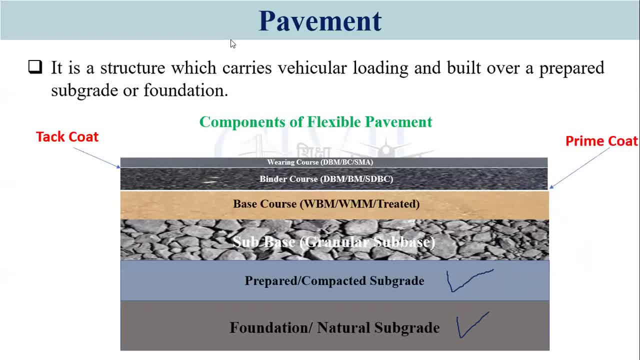 the compacted subgrade, whose thickness is 500 millimeter, that you have to keep in mind. then you're going to provide the granular sub base, which is for drainage purpose. then you're going to provide the base coat, Then binder course and finally wearing course. 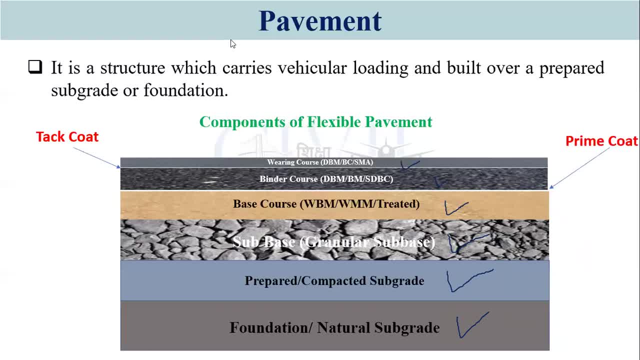 Now what you remember. in between a base course and binder course, or in simple words, in between a granular layer and a bituminous layer, We are going to provide a thin coat of bitumen for proper binding, That's what is simply called as the prime coat. 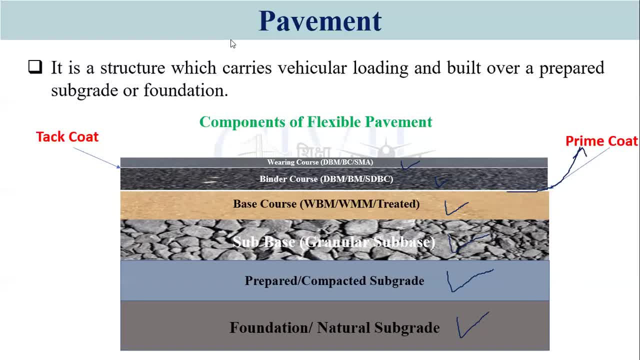 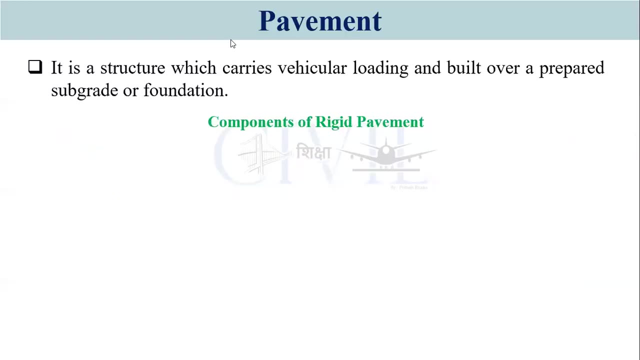 At the same time we again provide a thin bituminous coat between a bituminous, between two bituminous layer. That coat is simply called as the take coat. So this you have to understand In the case of a Flexible pavement. now, in the next slide we are going to talk about the various components. 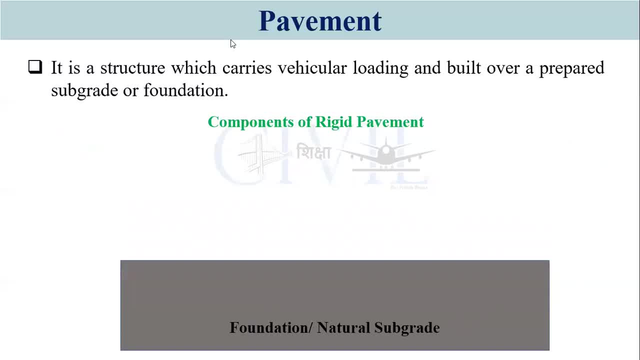 of the rigid pavement. So what we do have in the rigid pavement, again the compacted, also in the natural subgrade, which is constructed or prepared using parent material only wherever you're going to construct the pavement. After that we are going to have the compacted subgrade. 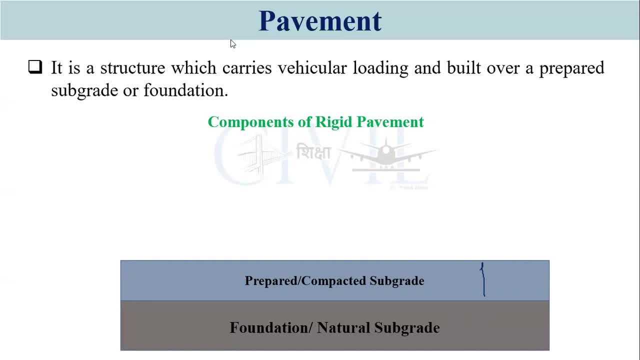 Why we have to provide this? because we want to increase the strength of the parent material. again over here, The strength and the thickness is going to be 500 millimeter only In the case of rigid pavement also, it is going to be 500 millimeter and the thickness of 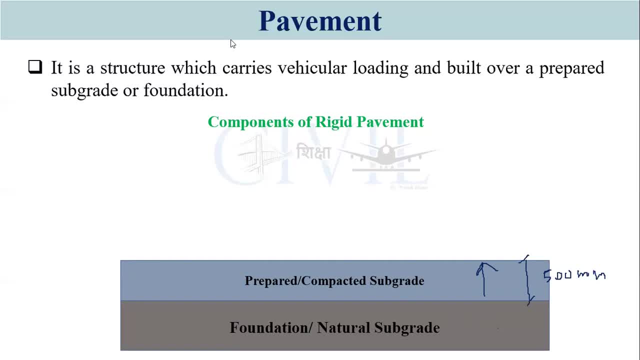 the bottom most layer, which is your natural subgrade, is going to be infinite, because you don't know up to what depth the layer is going, So it is infinite in depth. Then you are going to provide the granular sub base. again, it is for drainage purpose. 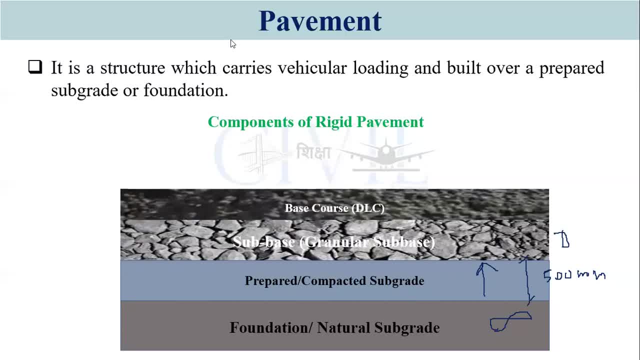 and after this, you are going to provide a cementitious base which is called as the DLC. The DLC means dried in concrete And it is a mix of concrete Whose strength is 10 mega Pascal, or the characteristic composition is 10 mega Pascal, or it is nothing. 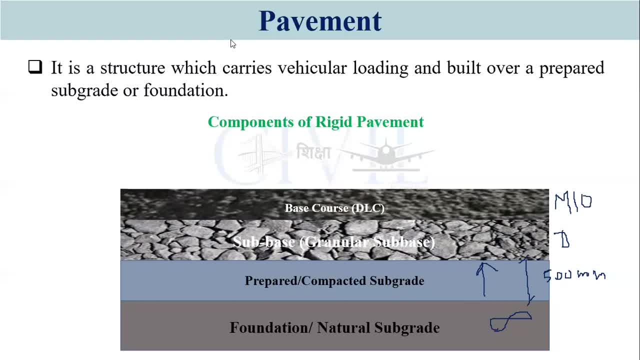 but it is a mix of M10 grade. And finally, we do provide the wearing course, which is simply called as the PQC means paving quality concrete whose strength is M40, which is specified by IRC 58. So you can see over here the number of layers are less as compared to the flexible pavement. 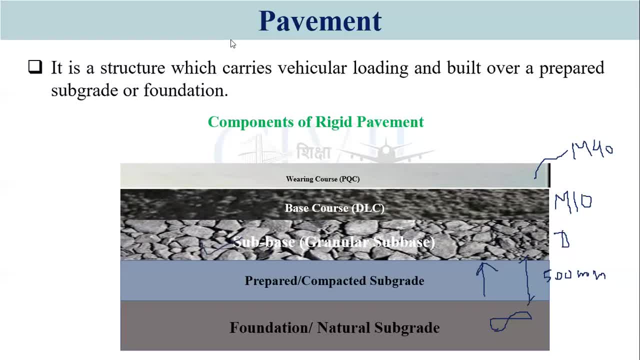 and over here what we have. we have the granular sub base. After that we are going to have the DLC, which is dry in concrete, and this is 10 mega Pascal, and finally we are going to have the PQC, which is paving quality concrete, and the strength. 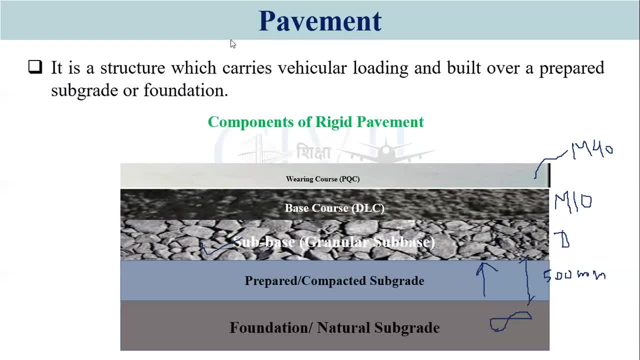 is M40. again like flexible pavement, We also provide one layer over here and the layer is called as the de-bonding layer. So in the case of flexible pavement we were providing the layer for binding, but here we are also bonding, but here we are providing the layer for de-bonding, because what we want 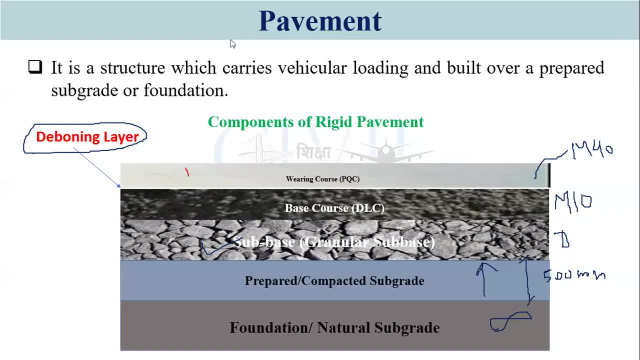 in the case of rigid pavement, That both of this layer, layer number two and layer number two, should move independently right. and to move them independently we don't want, we didn't want any bond in between. and to avoid that bond or say to prevent that bond, we do provide this de-bonding layer and 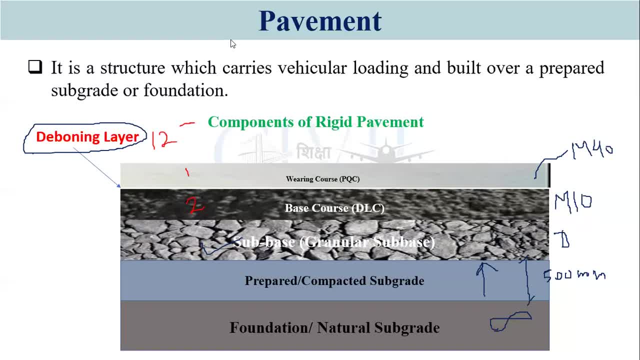 the thickness of this de-bonding layer is 125 microns. It is a PBL sheet which is generally available in market and the thickness of this layer layer is or the thickness of the sheet is 125 micron, which is also called as the de-bonding. 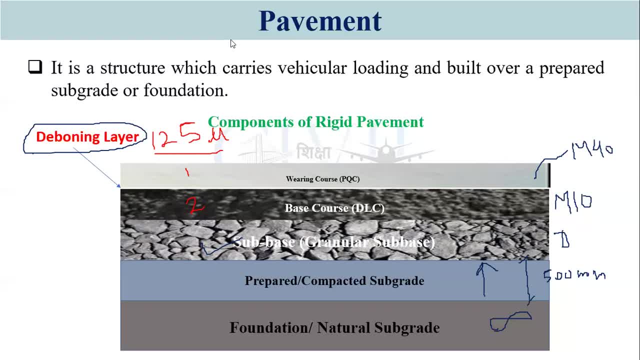 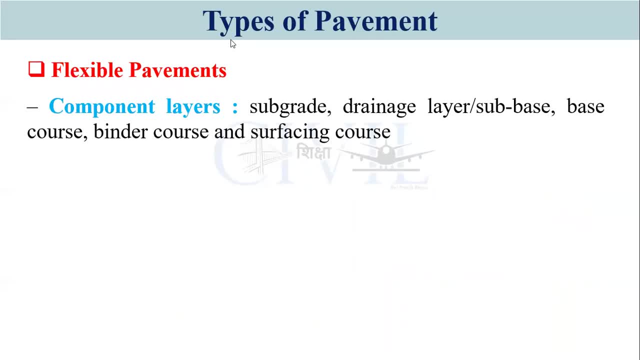 layer. So these are the different components of a rigid pavement and finally, you can see the slide again over where we are having the flexible pavement and these are the component layers that you have seen in the figure, and rigid pavement and these are the component layer, and sometimes you are going to provide the combination of these two, which is simply called. 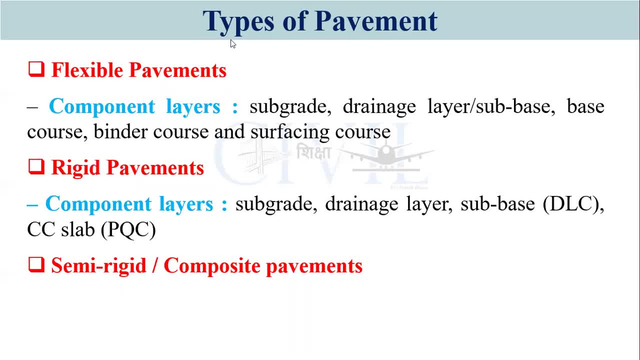 as the semi-rigid pavement or composite pavement. Now what you have to understand in the both of the pavement: in the case of the flexible pavement, the loader transfer is generally grain to grain, whereas in the case of flexible pavement, the loader transfer is through slab action. 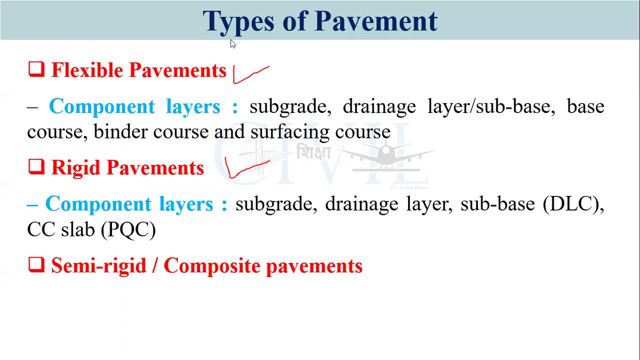 At the same time, the flexible pavements are flexible in nature, whereas the or say they have the good flexible strength, but in the case of rigid pavement, they have negligible or zero flexible strength. sorry, yes, flexible strength, but they do have the flexural strength which is required for the load transfer in the case of slab to slab action. 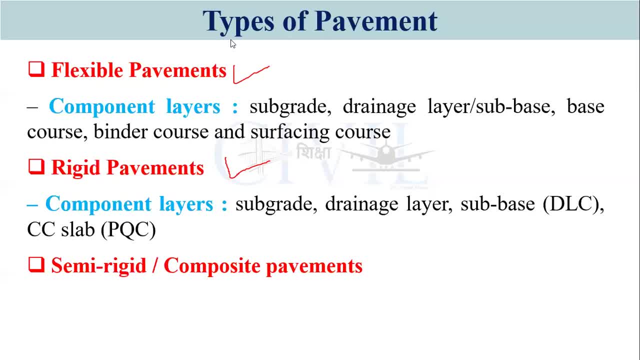 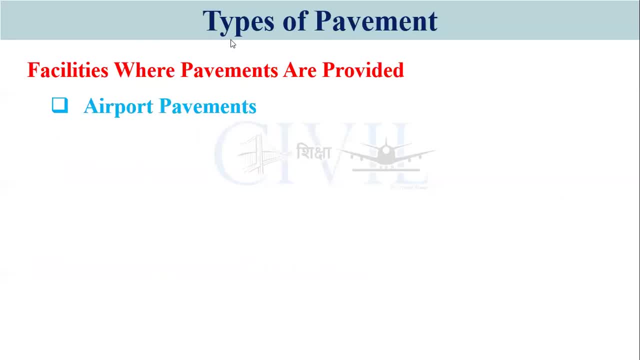 So these things you have to understand in the case of flexible pavement and rigid pavement. and finally, where do we provide this all type of the pavement So that you can see, say, the facilities where the pavements are provided? you can see the airport pavement, nothing but the runway and taxiway, then you can see whole road, same bus. 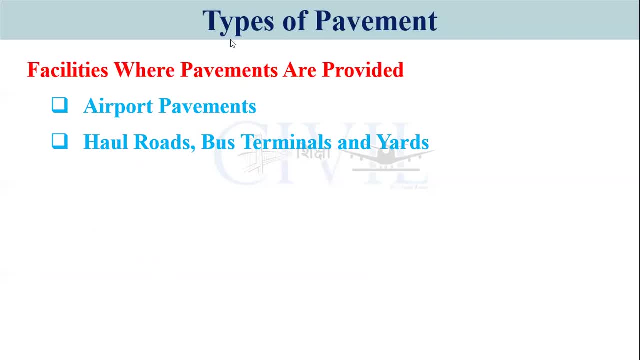 terminal and the yards over here. also, we are going to provide the pavement, then highway pavement, which is very common to everyone, that you can see the different examples over here- the national highway or express highway, then after that we are going to have the low volume road or say rural road, then we have the intersection area or urban roads and finally,